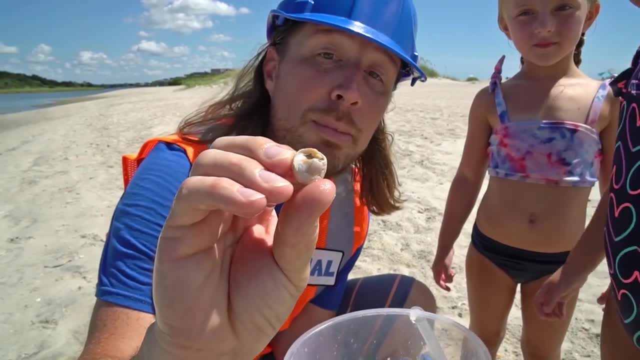 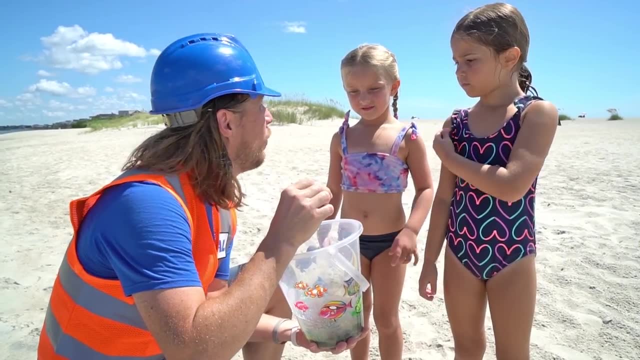 one's cool. You see that He's moving around in there. Oh, this is great. Oh, I have a great idea What. Let's build a sandcastle for him to play in. That sound good. Yeah, Oh, come on. 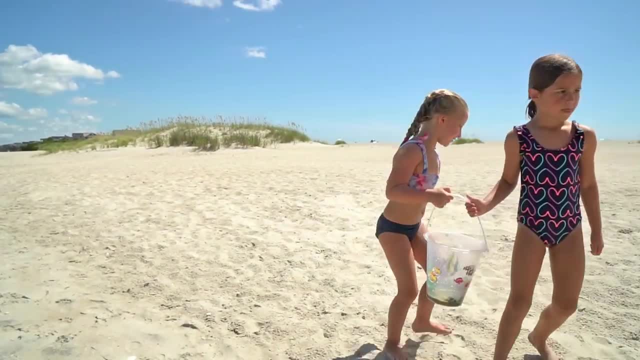 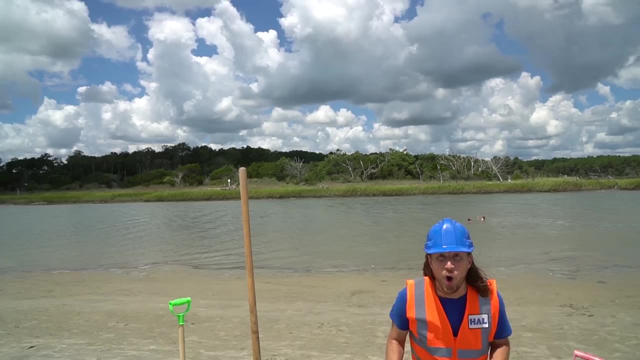 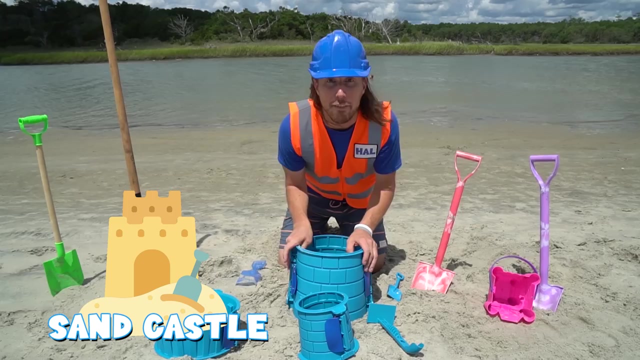 Here's that bag for you. Come on, Let's go. We are going to have an awesome day at the beach with my friends Elsie and Marla. Alright, my friends, We're going to get ready to build a sandcastle for our hermit crabs. This is going to be awesome. Have you ever built a? 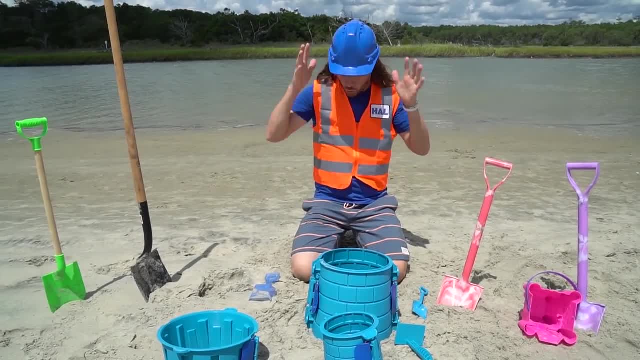 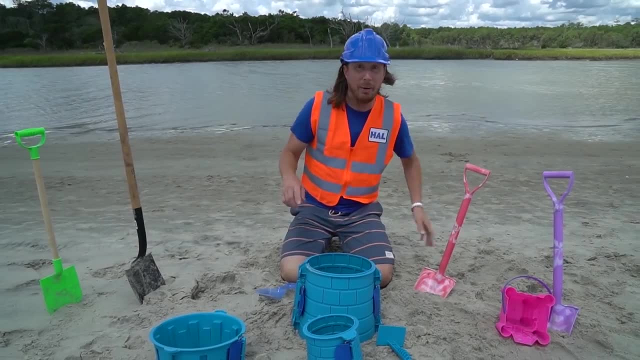 sandcastle before. It's really awesome. We've got all our tools here. We've got some really cool shovels. There's one there, Oh, that's a cool one. We've got some big ones here, Oh, and we've even got a real big one. This is going to be great. Oh, and we've got this. 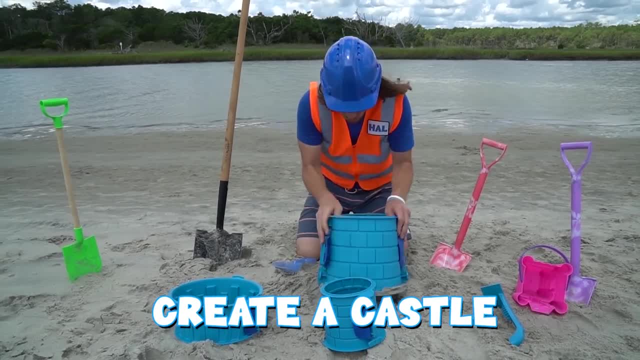 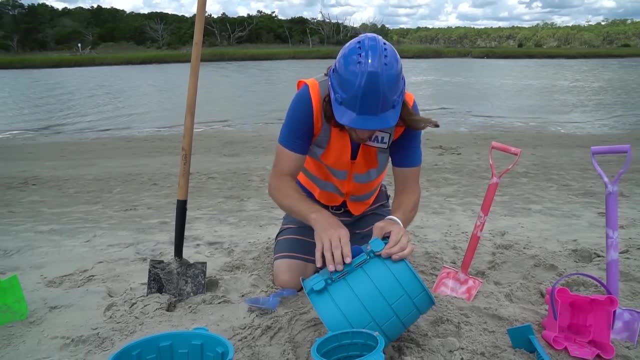 right here It's called Created Castle. It's a really cool tool. Let me show you how this works. We've got to put this together, just like this. We've got to clamp it together. Oh, we've got that one. Alright, there's the first one. Let's make sure that it's level. 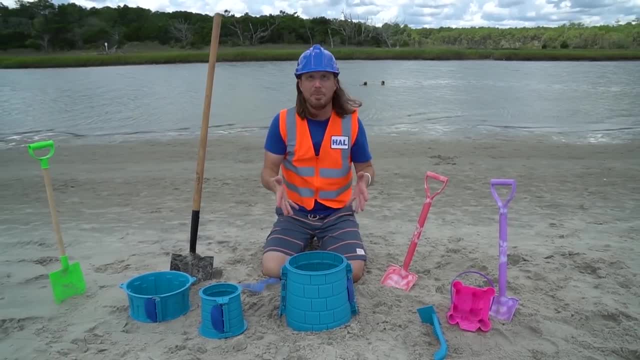 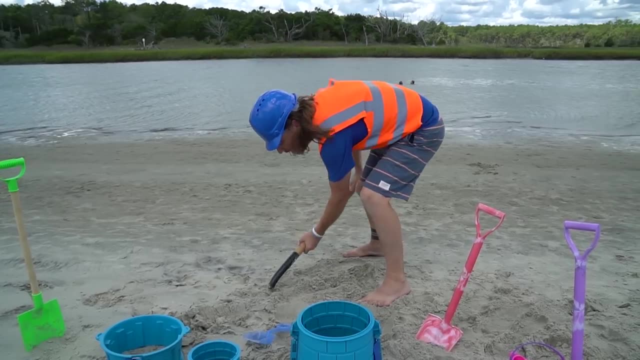 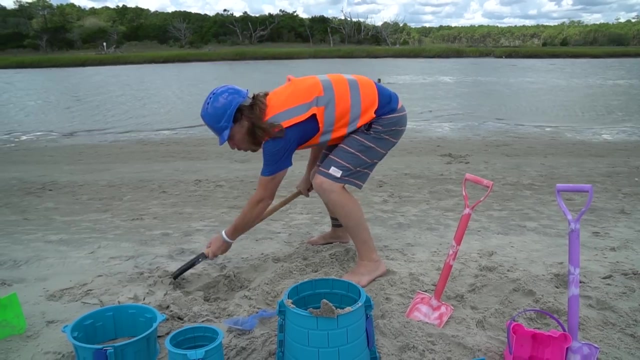 and then we get to stack those two on top. What's that? It's a big one. fill it up with sand first. all right, here we go. I think I'm gonna use the big shovel for this. here we go, one scoop at a time. oh, this is gonna be great. oh yeah. 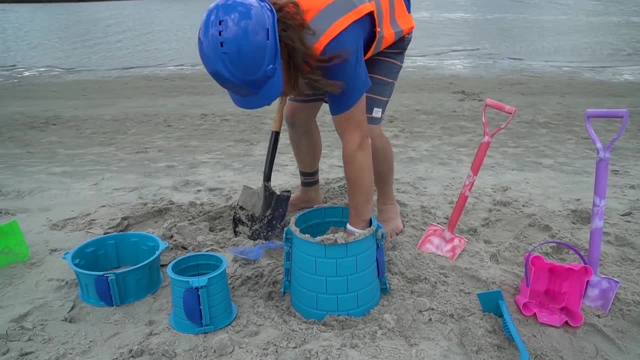 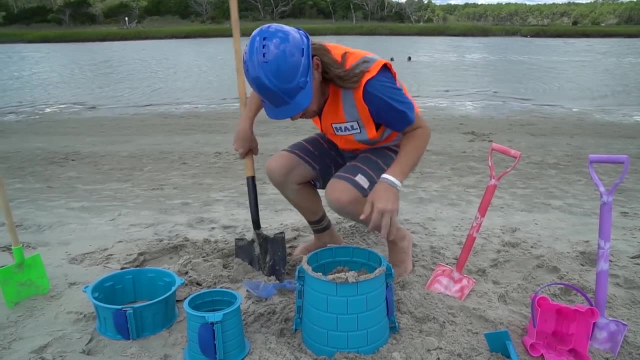 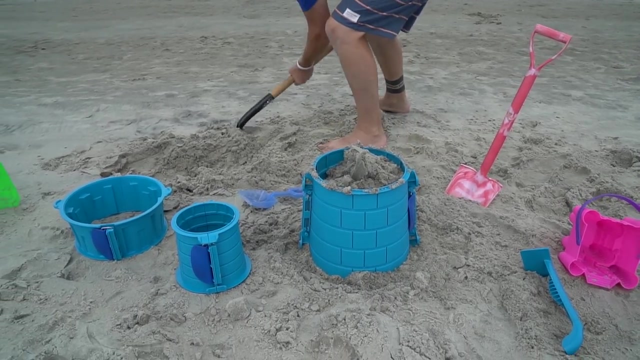 got to get it nice and full and we got to make sure we pack it down nice and tight so we don't want it to fall apart. get in there. really good, here we go. oh, that's great. a few more scoops here. oh, there's one there. oh, there we go all. 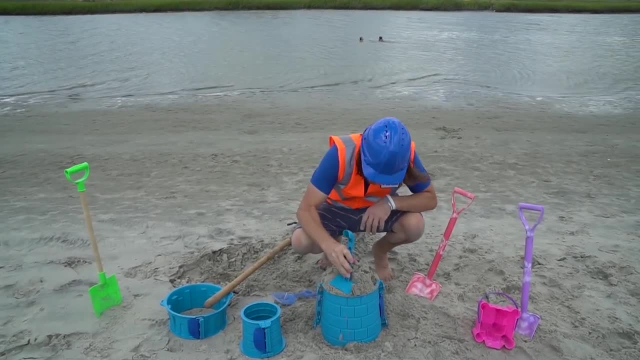 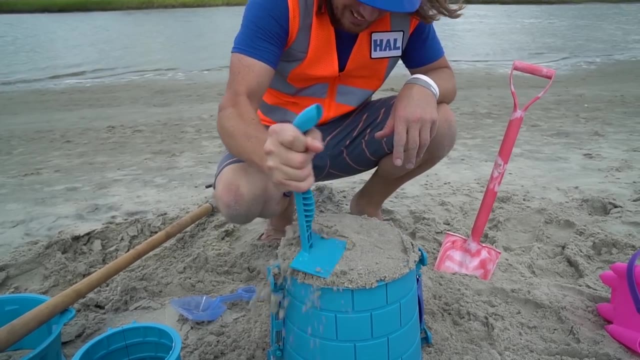 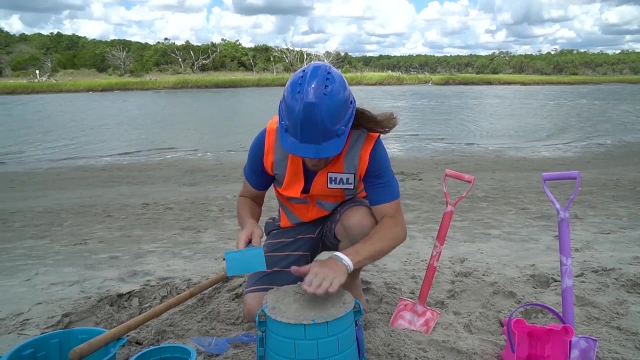 right, oh, let's see if we can use this right here to help pack it down. this is a pretty cool tool, right? oh yeah, it's got a flat edge on it so we can pack it down really good, really tight, and then what we can do is we can scrape off the 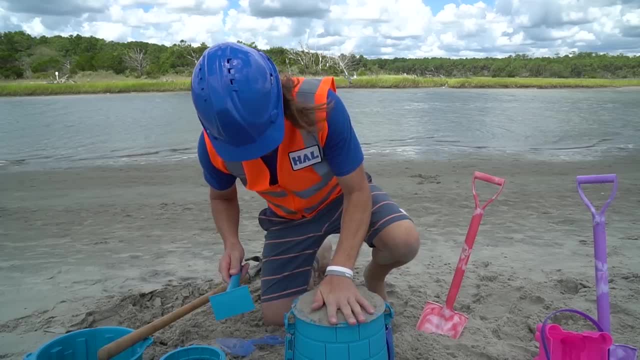 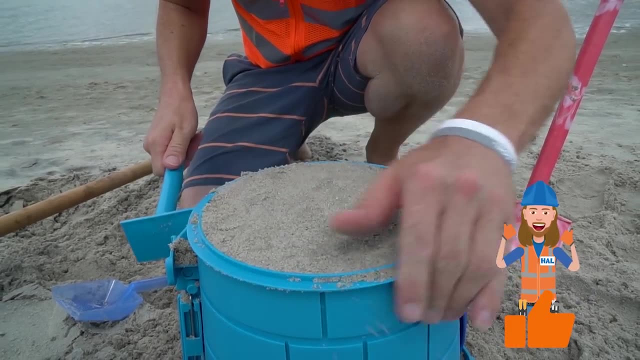 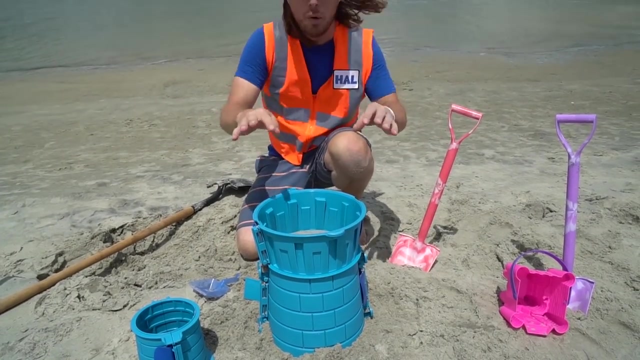 excess. make sure it's really good though. all right, here we go watch this. oh, we can make it flat, cuz you know why. you've got another part to put on just like this right here. check that out now we put the next one on. oh, come on, scoops in there. 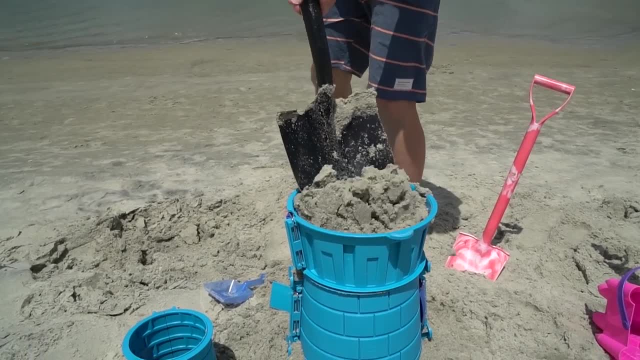 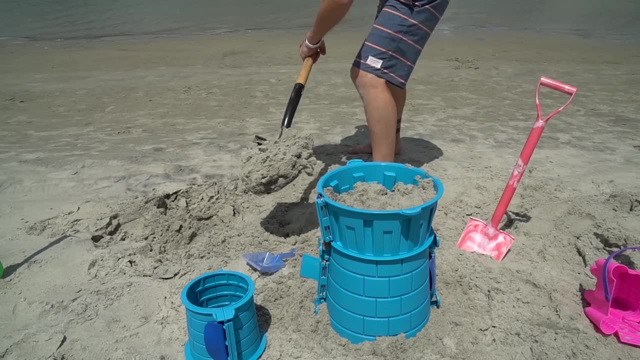 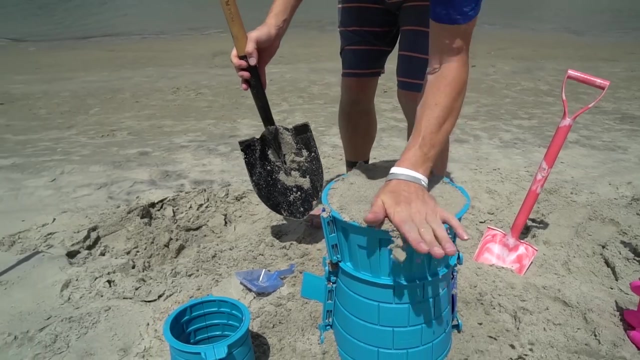 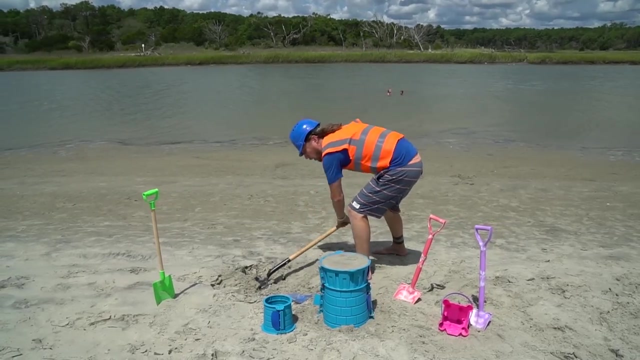 all right, here we go, fill it up. oh, let's make sure it stays on right. oh yes, this is gonna be great. alright, let's get it all nice and packed in there tight. let's see. oh, this is gonna look great. okay, here we go. maybe just a little bit more on there. 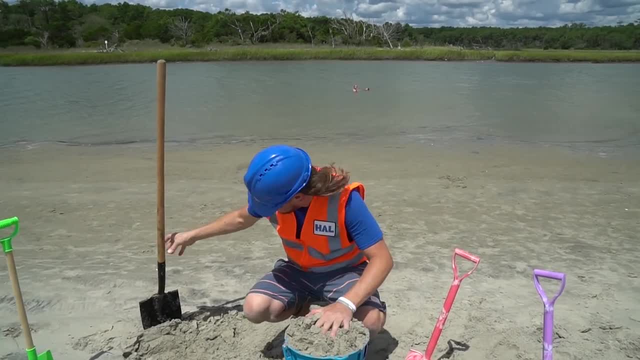 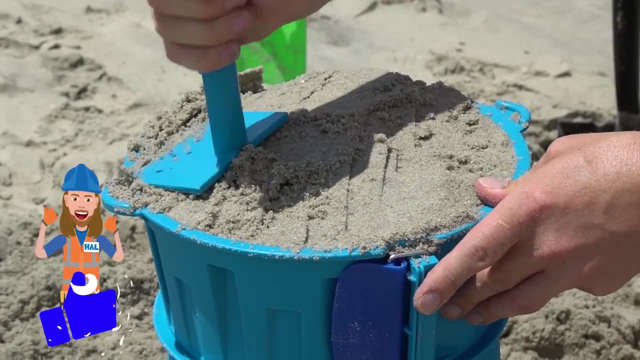 okay, yep, let's use our really cool tool to help pack it down. so we're gonna call this our packing tool. haha, that's great. alright, here we go, all right, here we go. All right, get it in there nice and good. Oh yeah, that looks really good. 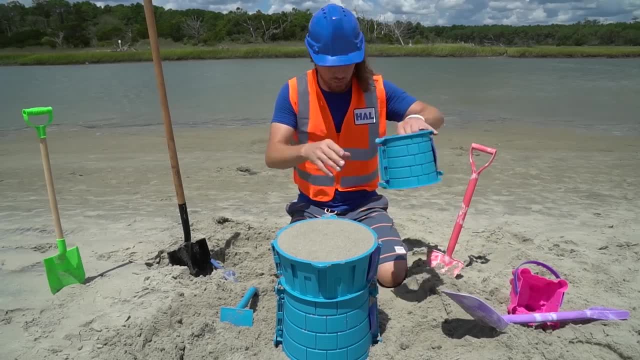 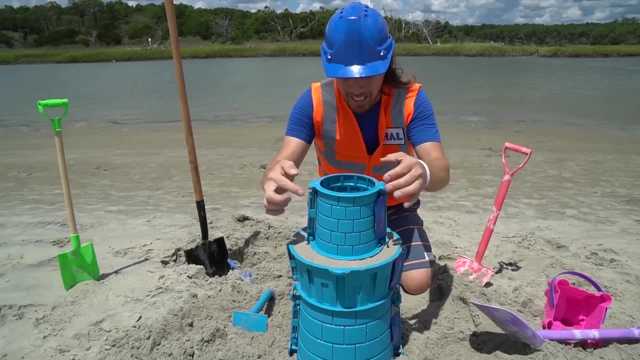 Really good for our last part here. All right, oh, and that's this one. Make sure we got it in the center. It's like building a house made out of bricks, but with sand. All right, so let's get a smaller shovel here. 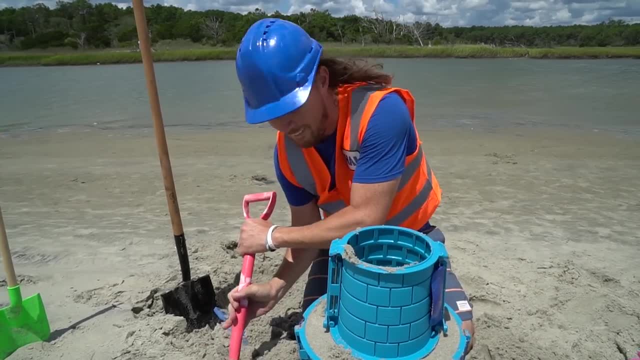 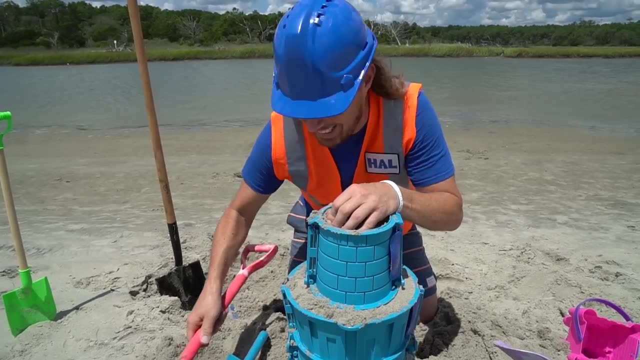 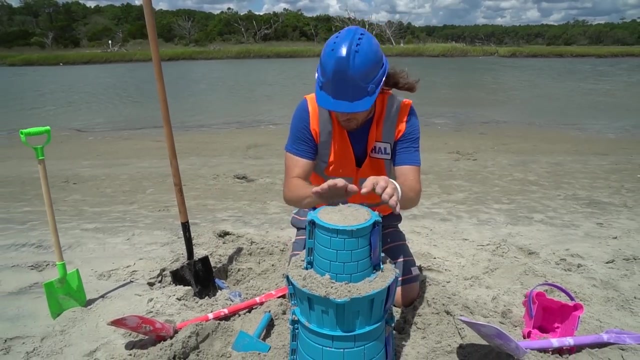 Let's fill this up with some sand too. Oh yeah, this looks like it's gonna be awesome. Oh yeah, these hermit crabs are really gonna like this. Oh yeah, here we go. All right, let's pack that in there, good. 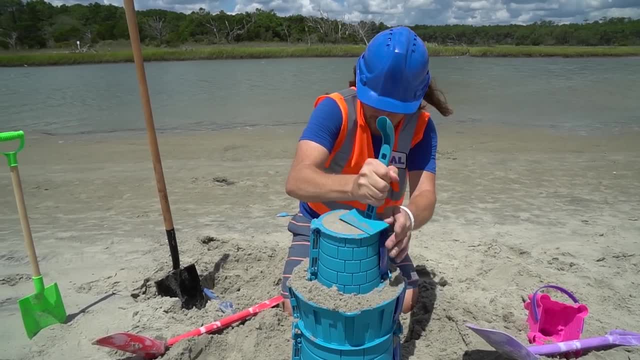 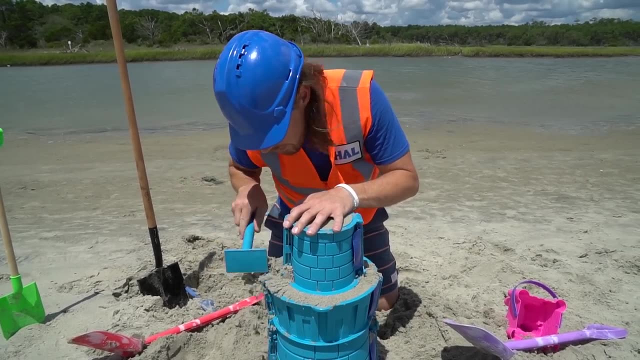 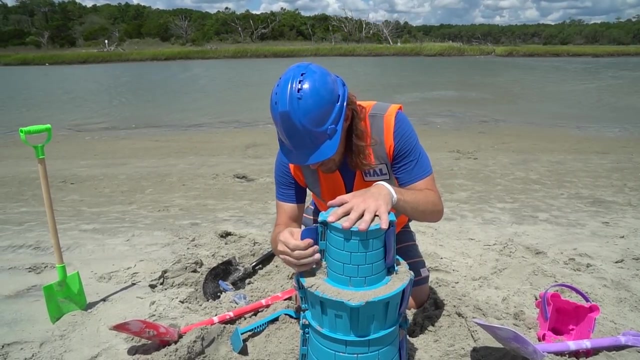 Get our packing tool. Oh yeah, here we go. Oh, that looks great. Oh, we can scrape off some of the sides here, Just like that, right there, All right, all right, Now let's open it up. What we have to do is open each side. 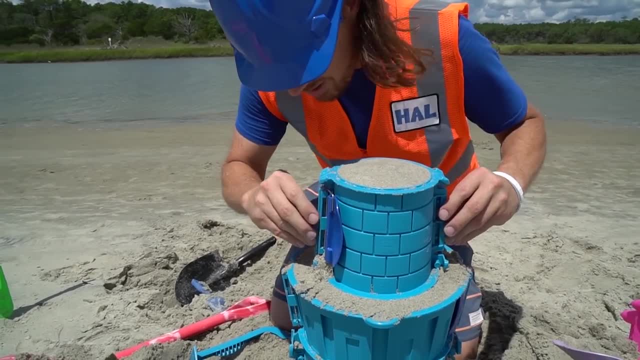 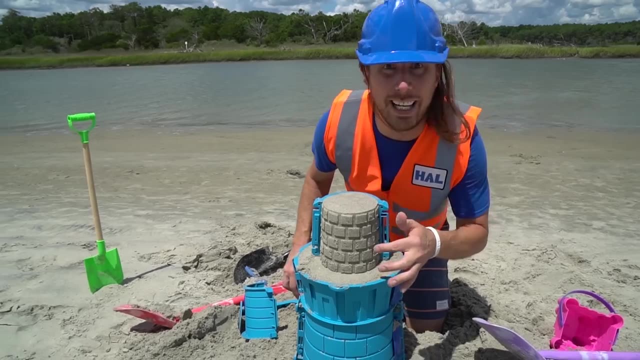 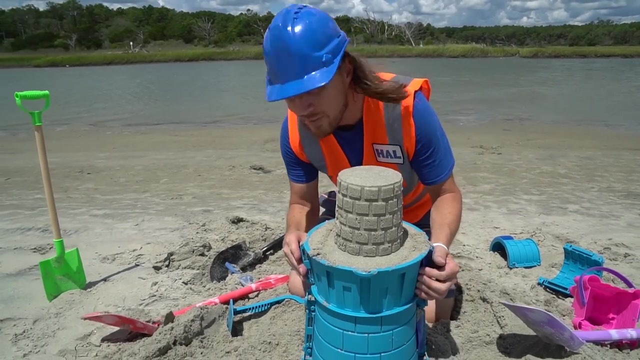 just like this right here. Are you ready? Here we go. Oh, let's see. Oh, wow, look, Looks like a brick wall. All right, let's get the backside off here. Oh, that looks amazing. Okay, now let's do the next level. 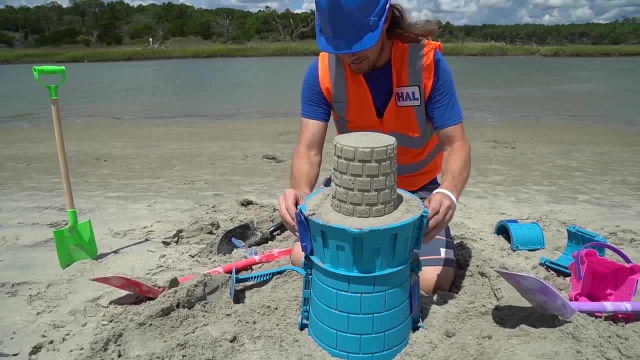 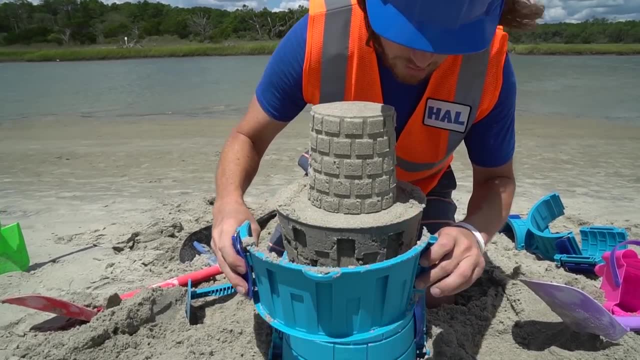 Let's unsnap it there. Unsnap it there. All right, let's see. Oh, we got this side off. Let's get the front side off. Oh wow, how does it look? Does it look good? Oh yeah. 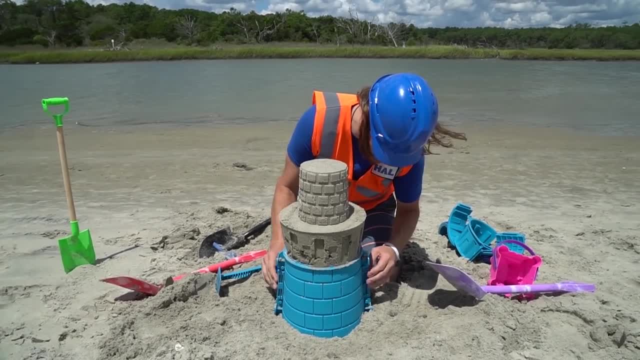 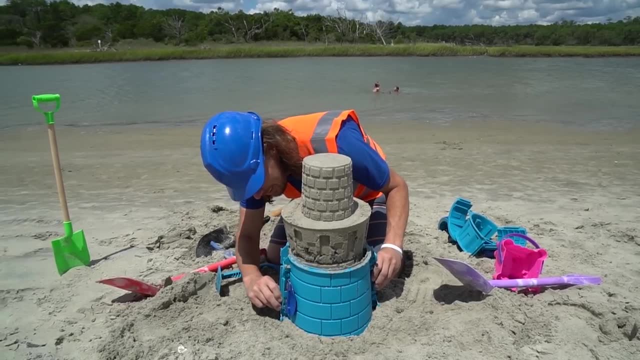 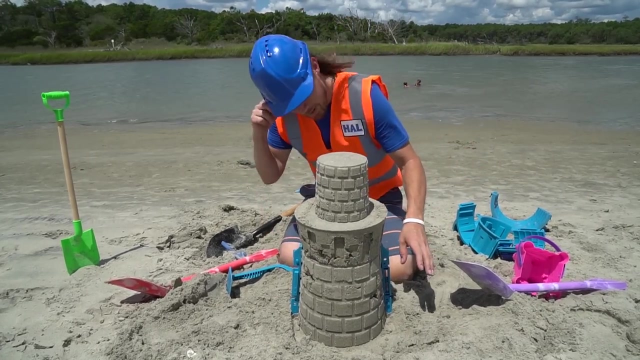 All right, now the bottom one. All right, easy does it, Easy does it. Oh, I think this is gonna be great. Slide it out of the way a little bit. Oh, wow, look at that. All right, let's try. 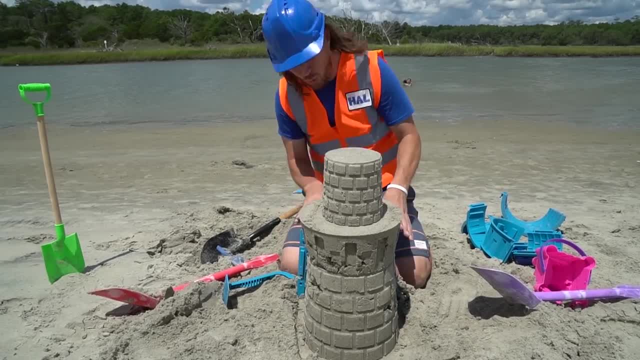 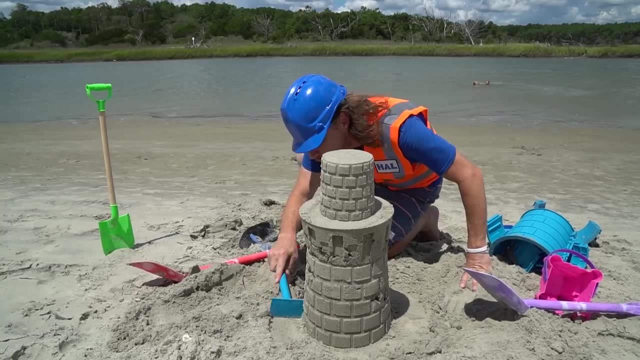 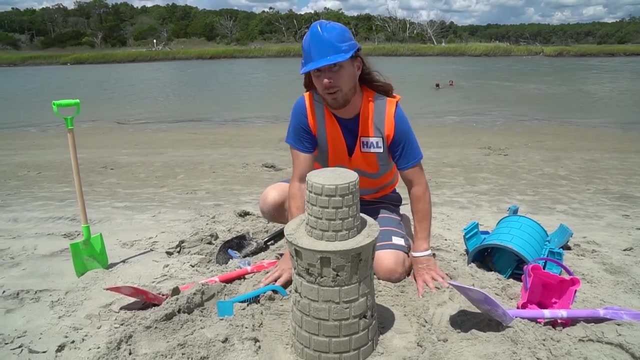 Let's try the backside here. Oh wow, look at that. Oh, this is gonna be great. Scrape around the sides here: Oh, that's amazing. Now we just need to get some shells to decorate it. It's gonna be awesome. 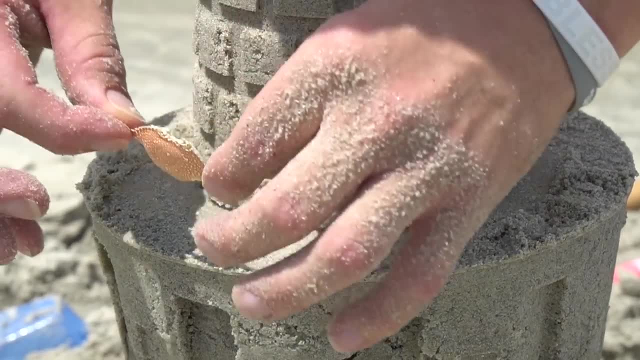 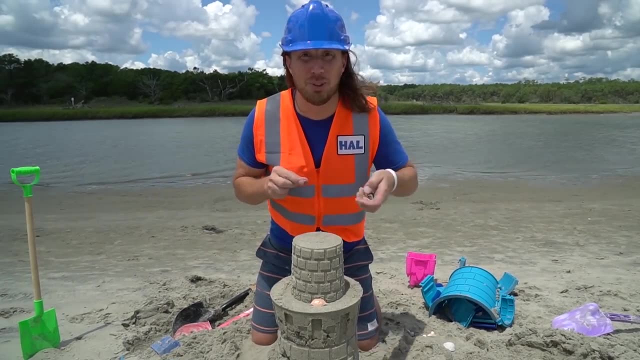 Come on, let's go. Look, I found this really cool crab shell. Let's put it right here on the top. Oh, that's gonna be great. Oh, we got some really cool shells here, Oh yeah, So let's put them around. 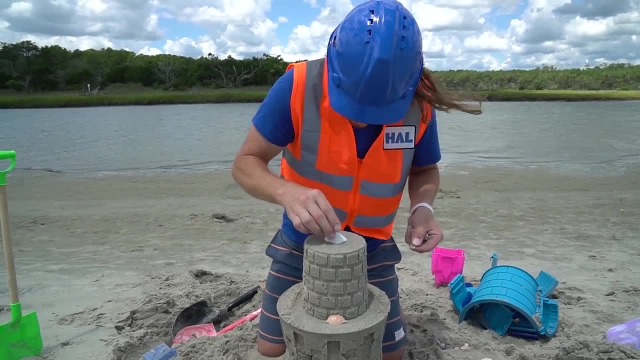 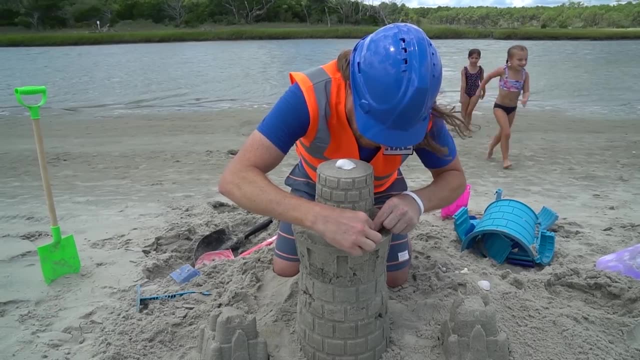 We got a big one here, Let's put it right on the top. Oh yep, This one's kind of a cool looking one. See if we can sit it right there. Oh, oh There, we go right there. 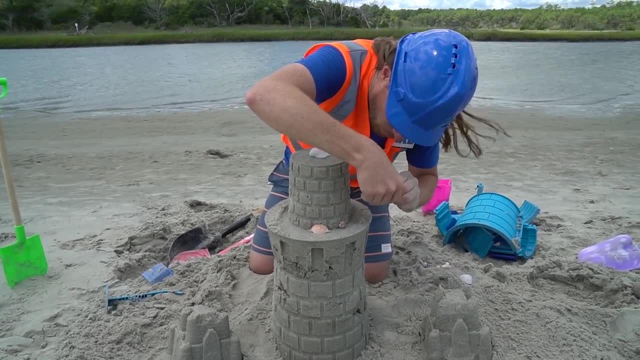 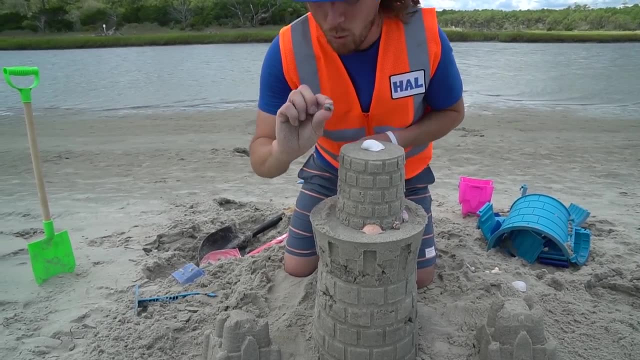 Oh, that looks great. Oh, there's one right here, Just putting them all around it, And whenever you decorate your sandcastle, you can decorate it however you'd like. That's a cool looking shell right there. That one right there. 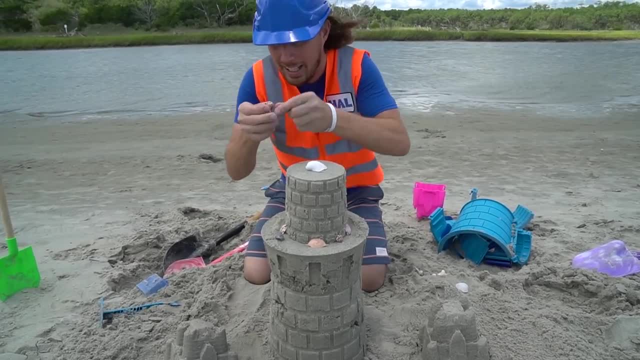 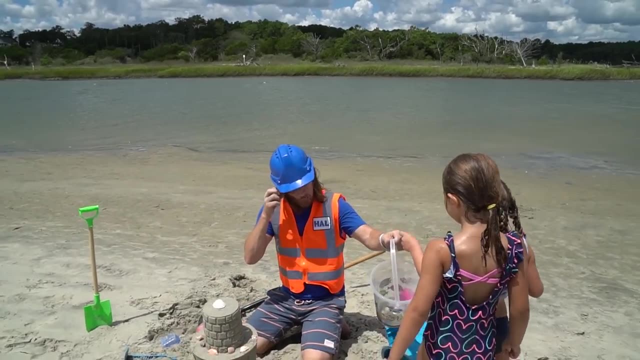 These are cool. That one there. Look, It's like a little teeny, tiny conch shell. Here's how we found some more. Oh wow, That's awesome. Let's see what you got. Oh yeah, Oh wow. 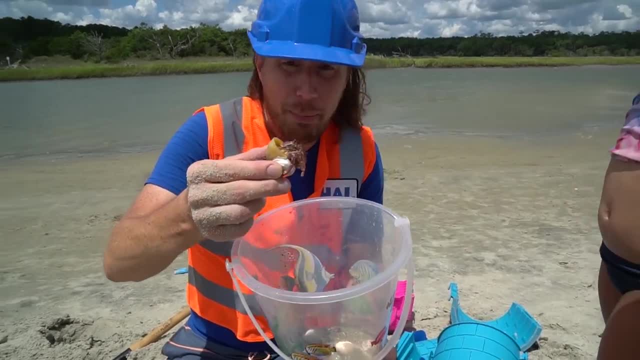 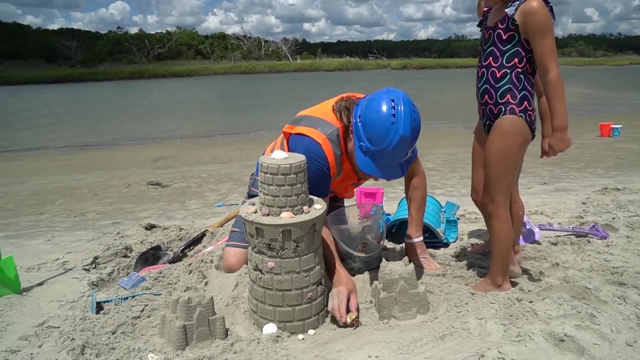 These are big ones. Check that out. Oh, that's a big army crab. Oh well, we got the castle all decorated. Let's see if we can set them out. We'll set the big one right there. Check it out. 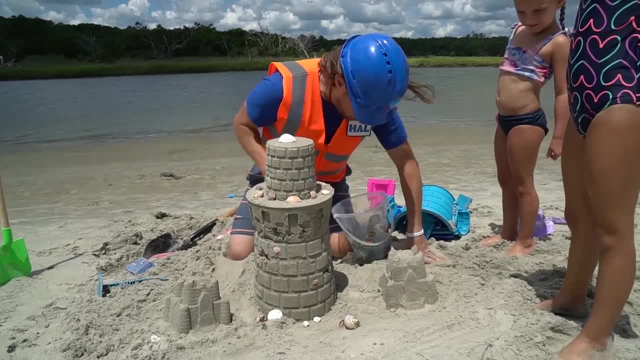 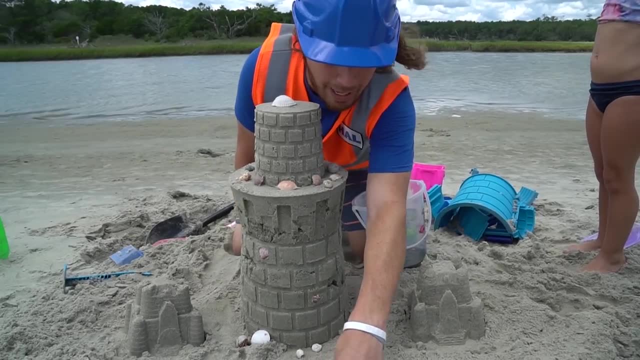 Oh, there's one right here. Oh, they're already moving around. They must really really like it. And then we've got some right here. We're gonna set them on the top. He is moving Here. we'll move them back. 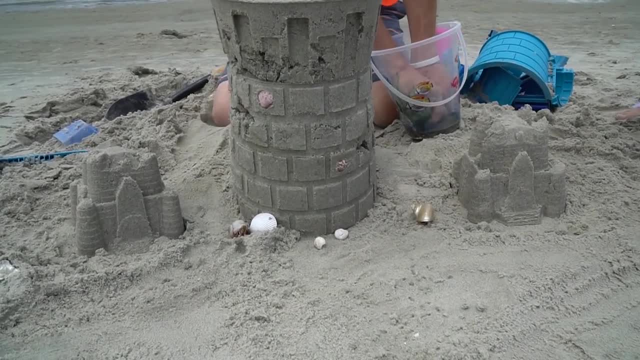 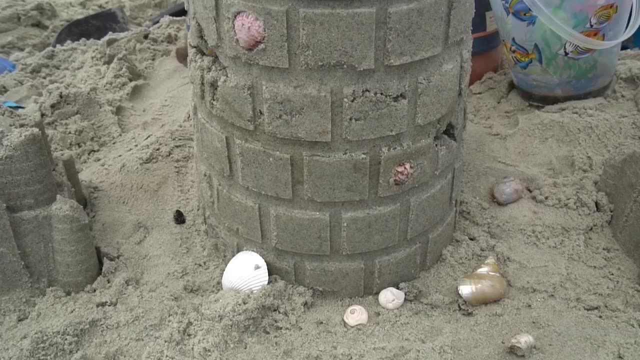 How about that? We'll move them back right there. Okay, Oh, we got some right here. Oh, we set them on the top. Oh, that'd be cool. It's like they're looking out. Whoa, There's a crab shell right there. 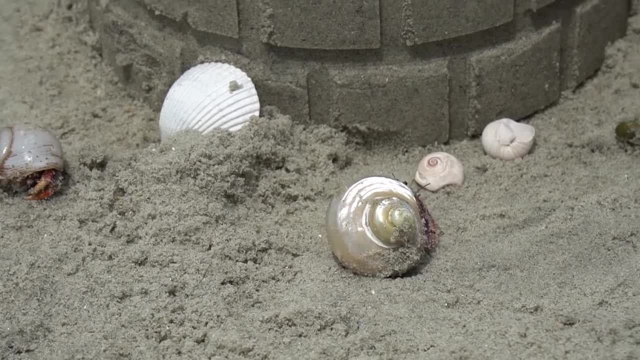 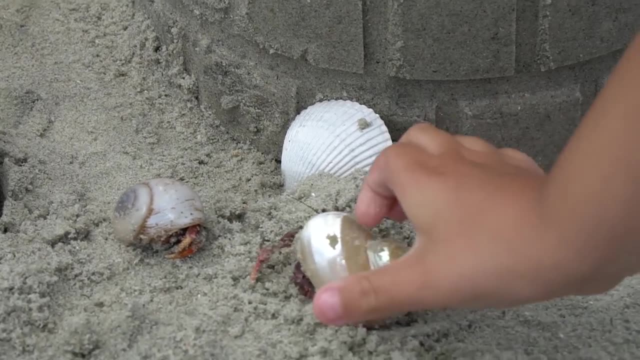 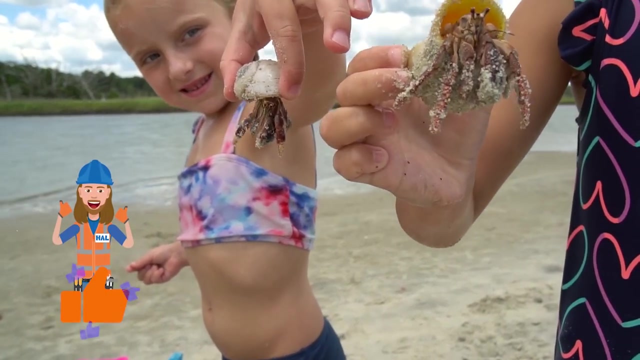 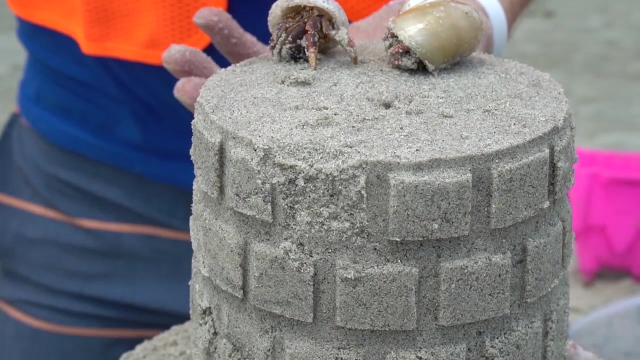 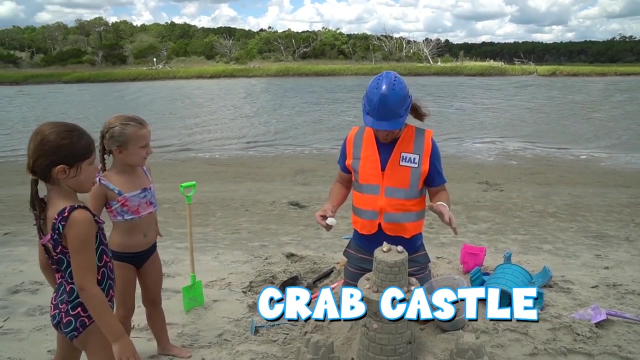 You see it, We can call this the crab castle. That would be totally awesome. Oh, it's a crab castle. All right, Here we go. I'm gonna go ahead and put this one down here. okay, Crab castle, Oh yes. 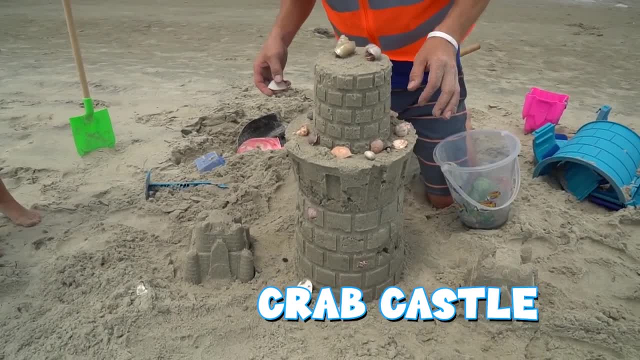 It's the crab castle. We're having such an awesome day at the beach today, right Yeah, We have a lot of food. We're having a lot of fun. Yeah, Yeah, Yeah, Uh, huh, Yeah, Yeah, Yeah. 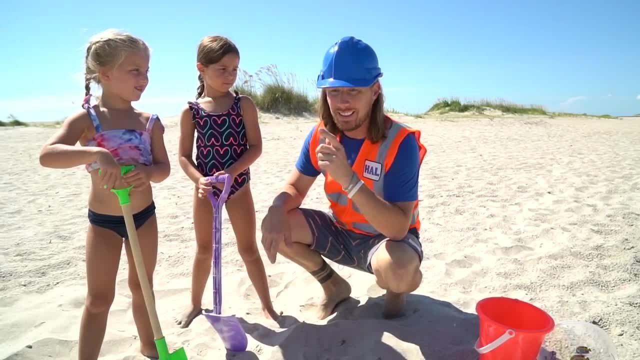 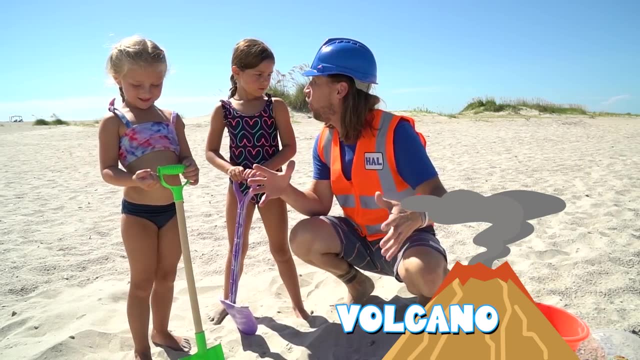 But you know, I have a really awesome idea. I think maybe we should build like this humongous mountain. Maybe we can turn it into a volcano. Does that sound really cool? Yeah, Oh, that sounds awesome. Okay, so this is what we need. 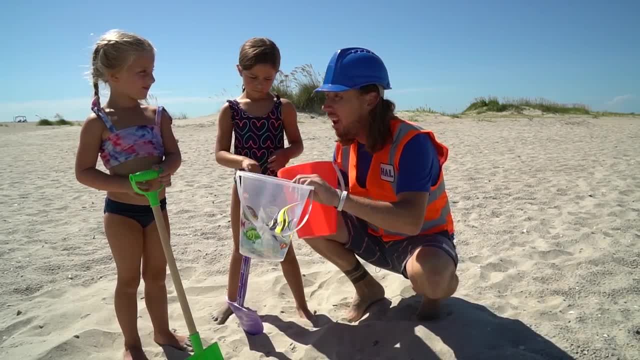 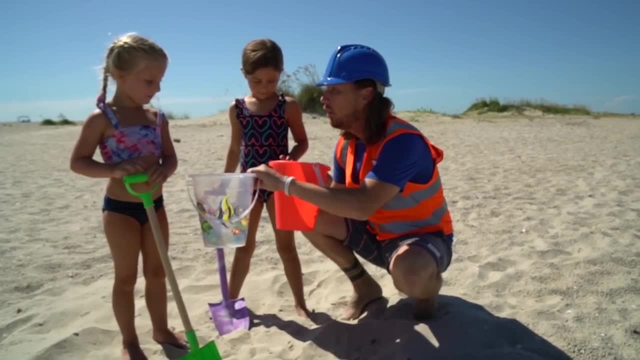 You've got shovels, Oh, so we need a bucket, We need lots and lots of sand. So you guys take each bucket and y'all go fill it up with sand and y'all bring it back to me. Okay, You think you can do it. 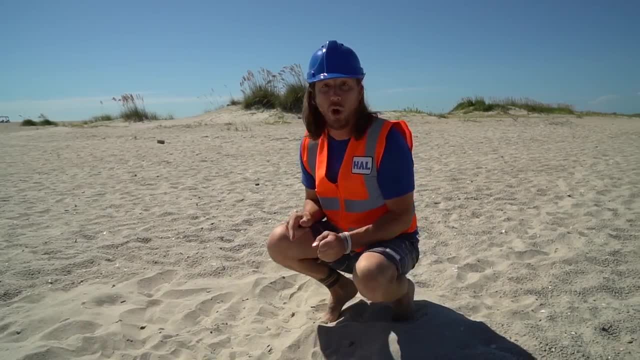 All right, here's your bucket, here's your bucket, And y'all can go right over there and fill it up with sand. Oh, this is gonna be great Cool. And I need one really important thing: This is a really cool PVC pipe. 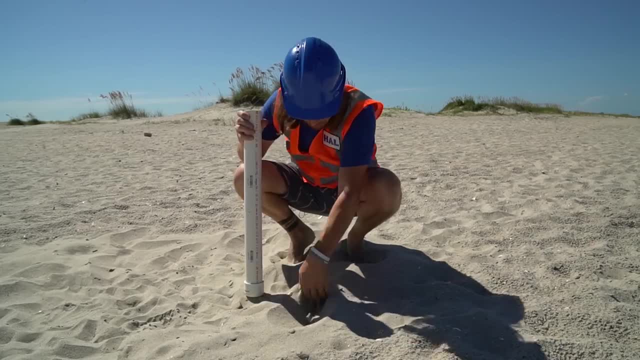 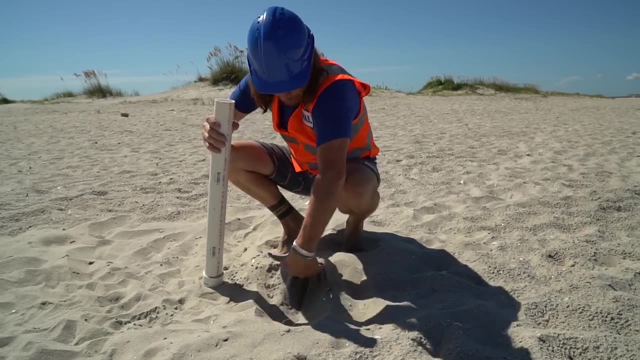 I'm gonna put it in the ground and this is how we're gonna make our volcano. We need a big hole here. Let's see, Get in there. There we go And as they bring, let's see a little bit, a little bit, a little bit. 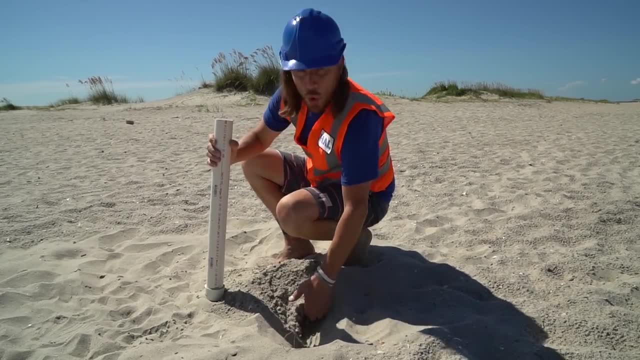 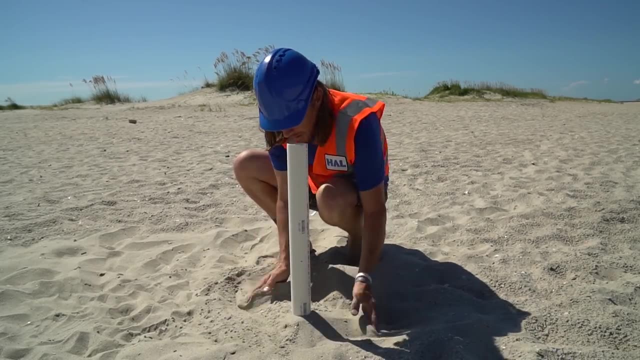 And as they bring the sand, we'll pile it up like a big humongous mountain. Oh yeah, this is gonna be great. That's a perfect start, right there. Think so, Right, Ha ha. Now we just gotta wait on some sand. 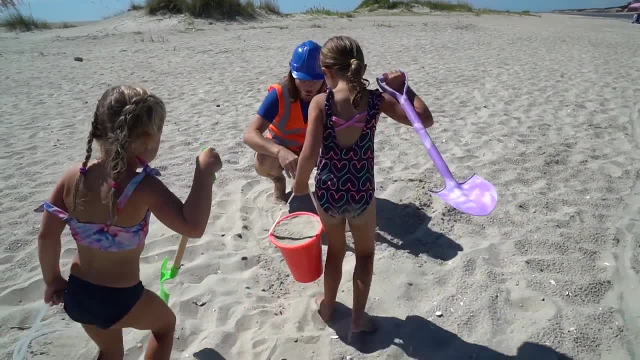 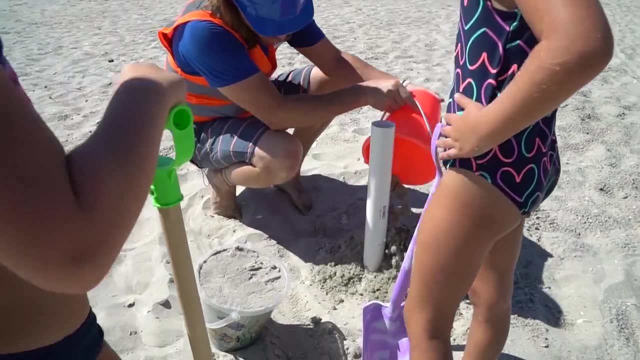 Look, here comes some sand and my helpers now. Oh, oh, that's great, girls, We got one big cute bucket here Here. let's see if we can dump it. Oh, that's great, Here's your bucket back. 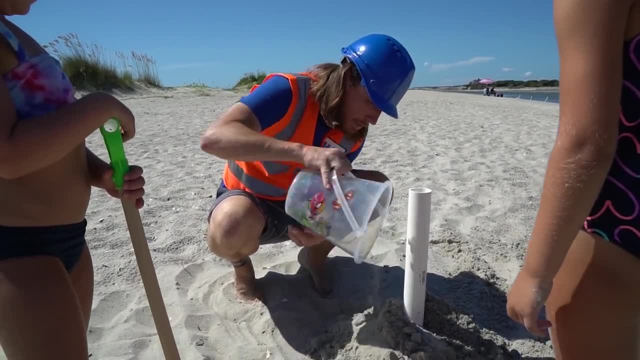 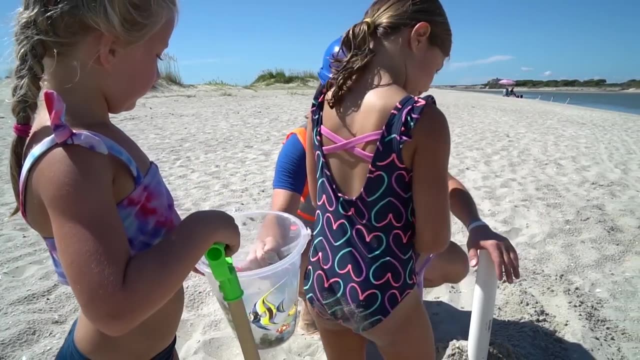 All right, let's dump this one right here. Oh, y'all see this PVC pipe right here. Oh, it's gonna be a really cool trick later on once we get all our sand around it. So here's your bucket. Let me get your bucket. 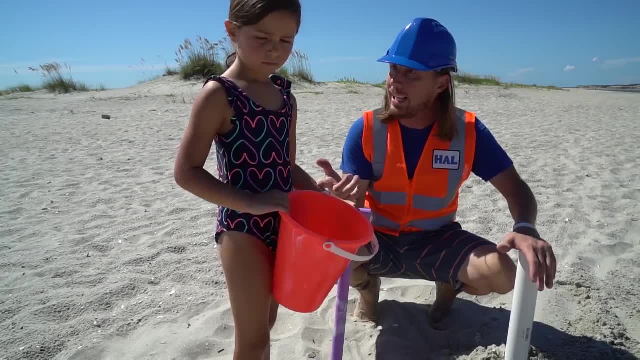 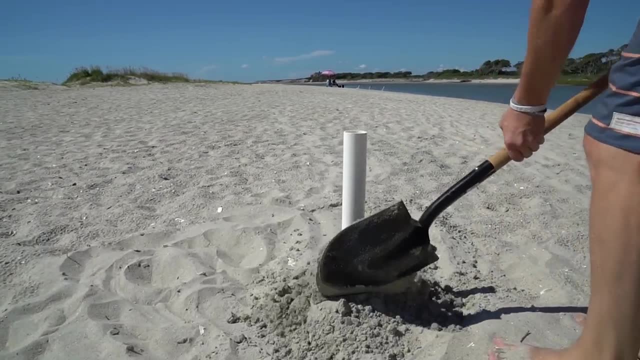 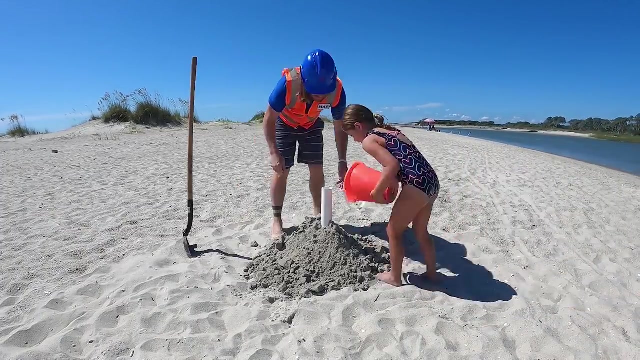 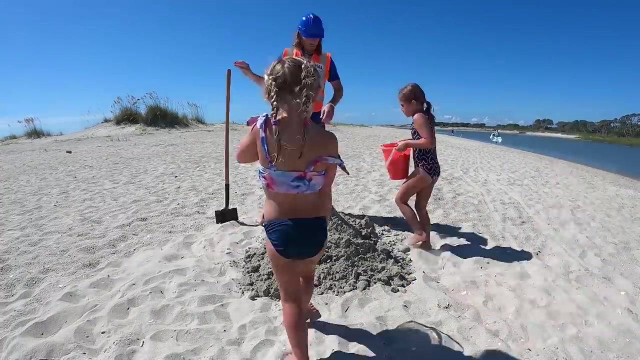 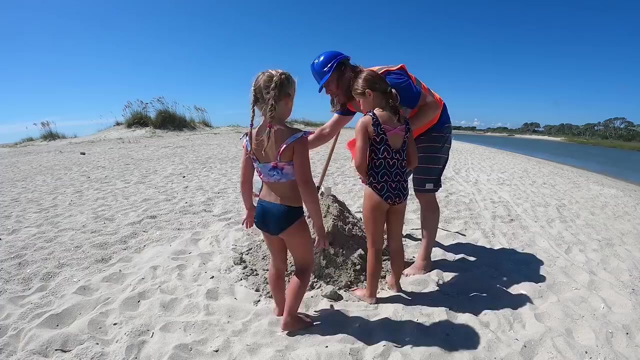 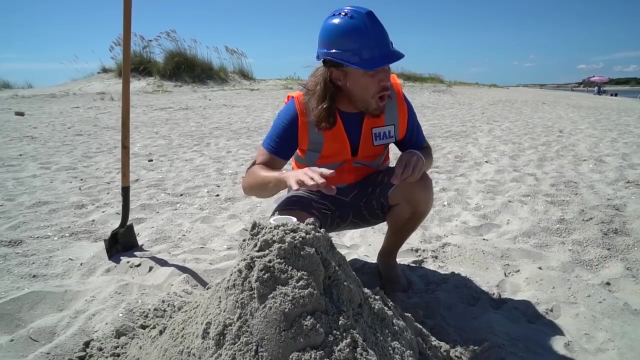 I think we need some more sand. Oh, I might need to get a shovel and a bucket to help you guys out. Come on, let's go, Let's go. Oh, wow, here we go. The last few buckets. Sit that right there. 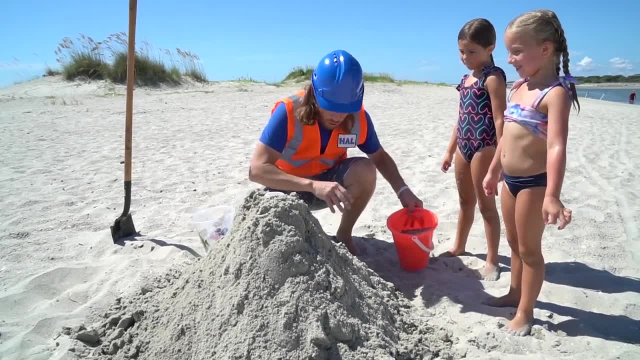 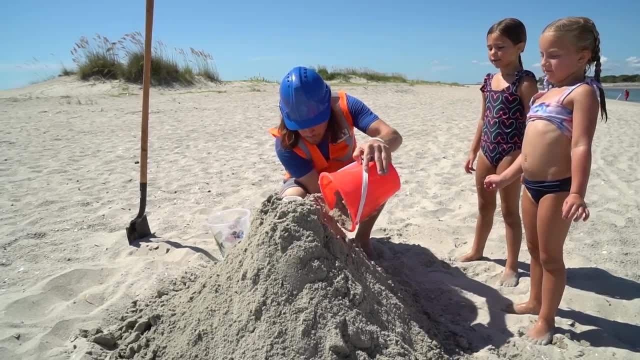 Oh, wow, Girls, we work really really fast, don't we? Oh, this is gonna look great. This is gonna be great. All right, last bit here. Does it look like a mountain? Yeah, That looks like a cool volcano, right. 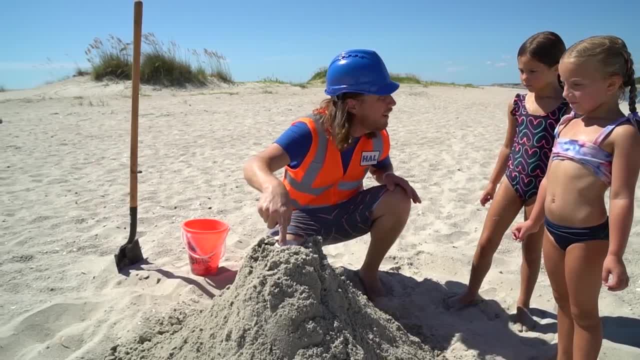 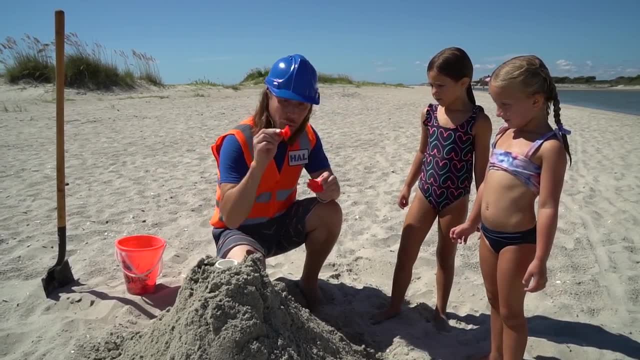 Okay, all right. So we got all of that in there and you see the pipe right there, right, All right. so we got some really, really important things. First off, safety. first, We gotta put out some safety cones to make sure nobody goes anywhere near it. 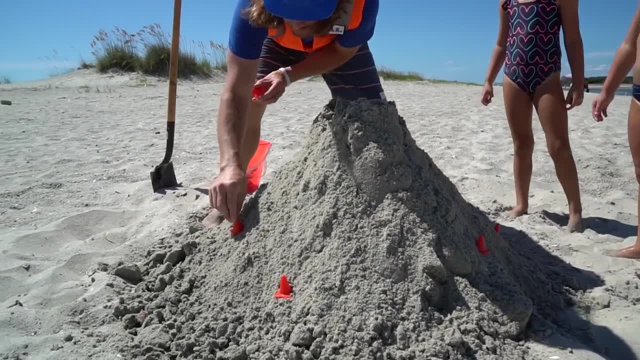 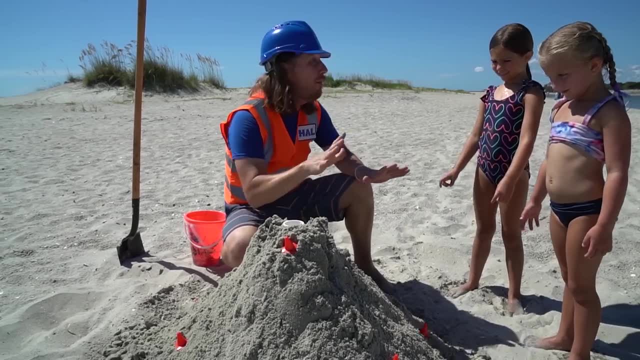 All right, we'll put one there. We'll put some up here right here, right here. Oh, maybe we might put one right there, so, nobody knows, it goes to the top right When it erupts. oh yeah, All right, so we have two really important ingredients. 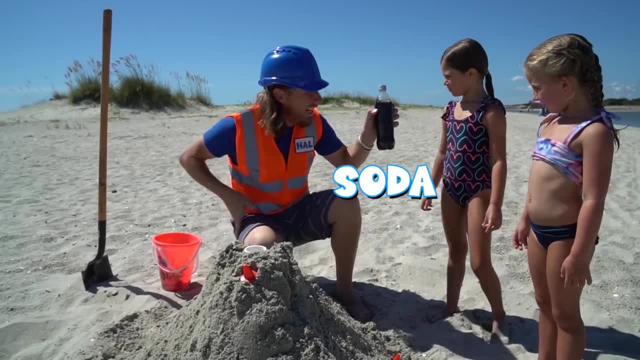 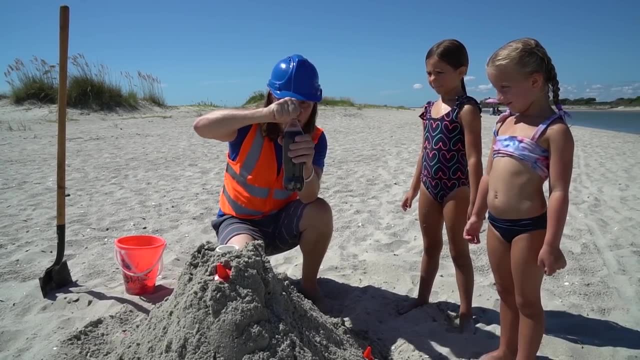 First is some soda. Oh, you like soda? Soda's really good. All right, here we go, let's see. Oh, you hear that. Oh, look, it's even got some bubbles inside of it. I really think that those bubbles are gonna help. 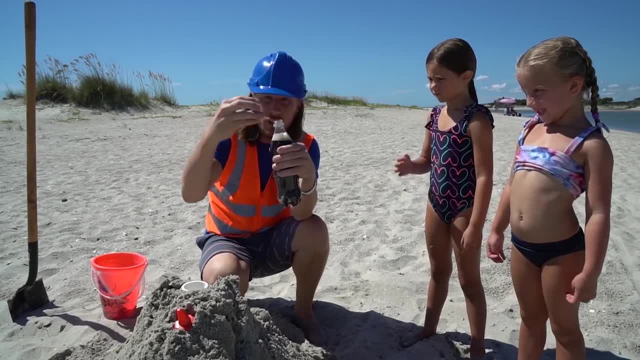 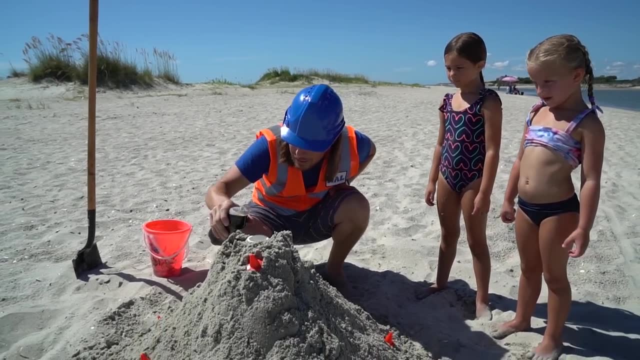 with the explosion. All right, so you wanna hold onto the cap? for me Gotta make sure that we don't let any trash go on the beach. We're gonna pour a little bit of soda right into our pipe. Can you hear it fizzing in there? 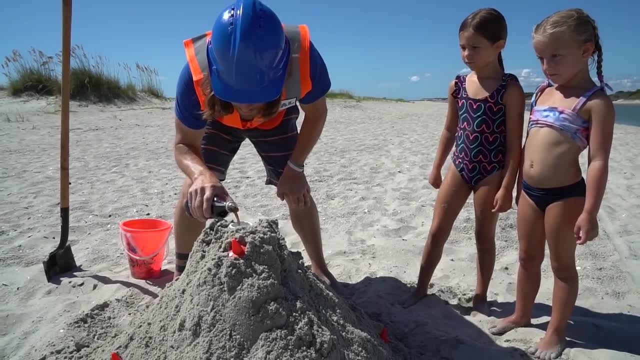 Oh, yep, here we go. Let's see, Almost almost. I think we should fill it up to about right there, Girls, what do you think's gonna happen? I think it's gonna explode. Explode, You think. 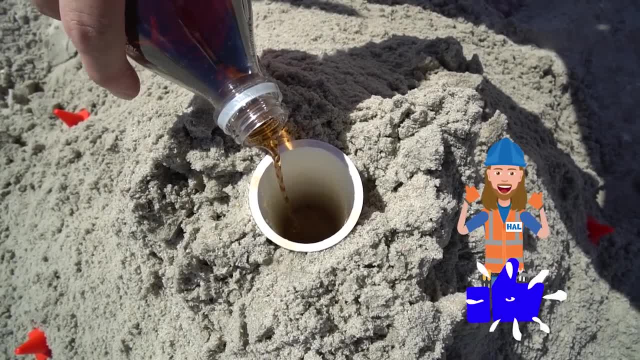 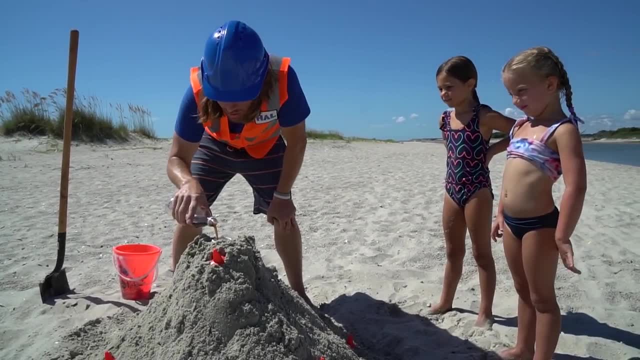 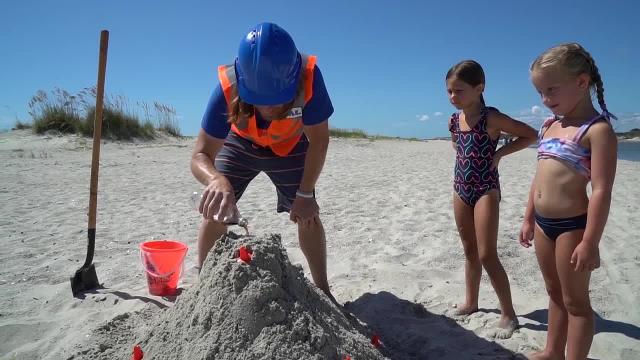 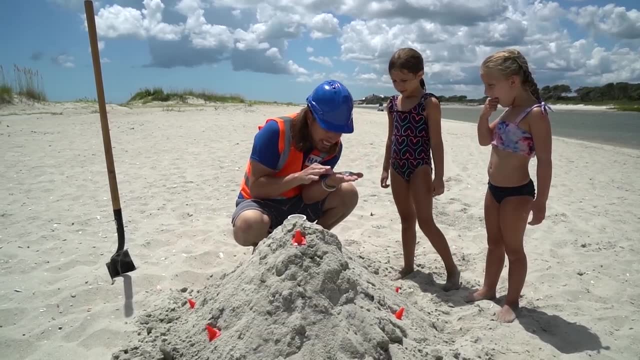 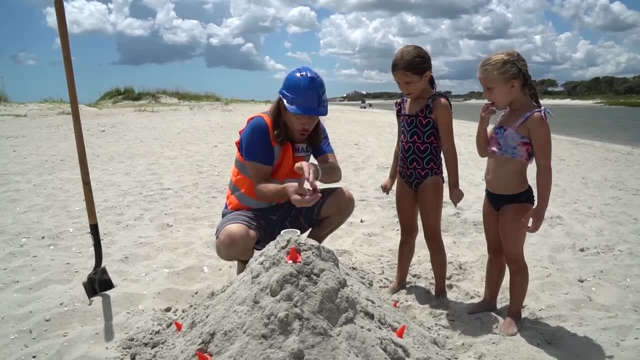 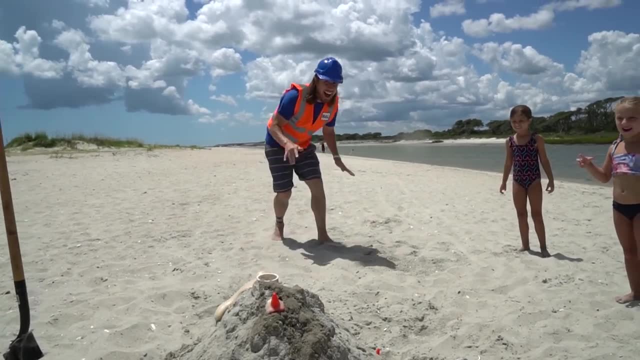 Oh, you feel the earth shaking. Here we go. You might wanna watch out. Whoa, Wow, Oh, and it's using them the sides. That was awesome. It's the beach volcano. I'm out, I'm out. 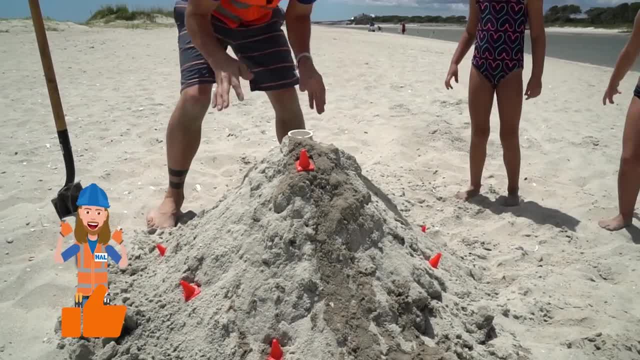 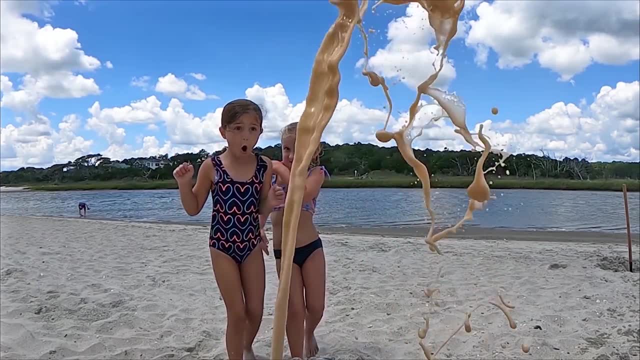 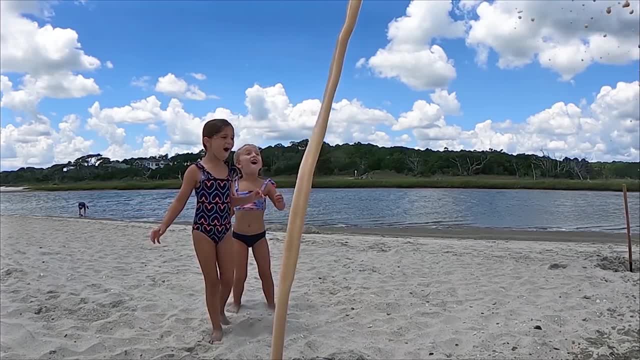 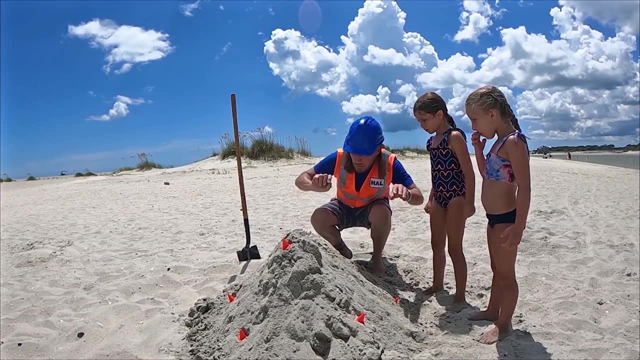 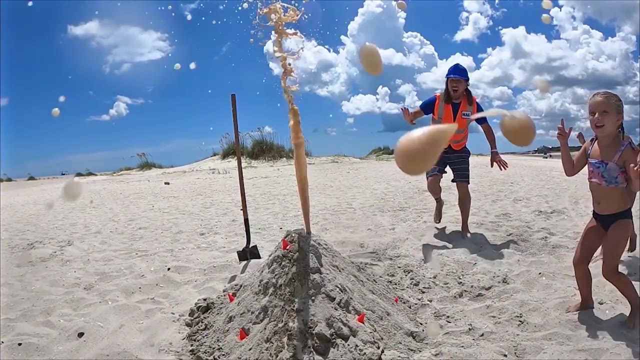 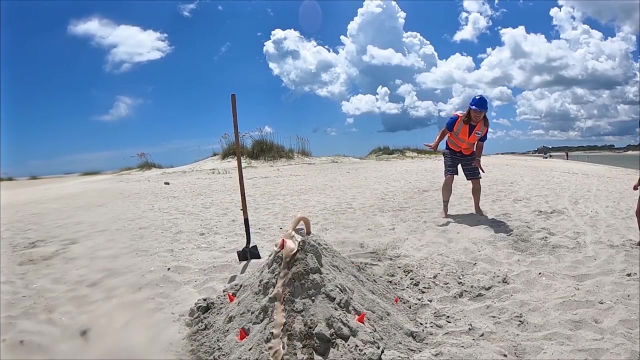 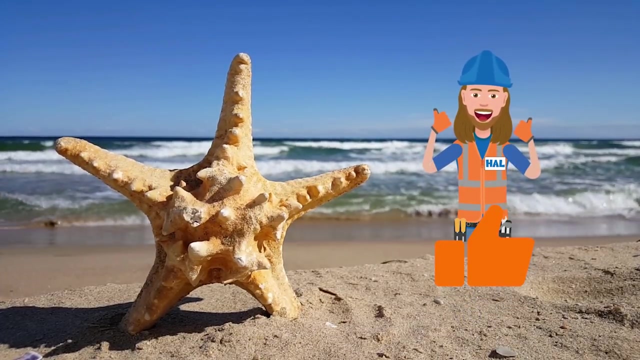 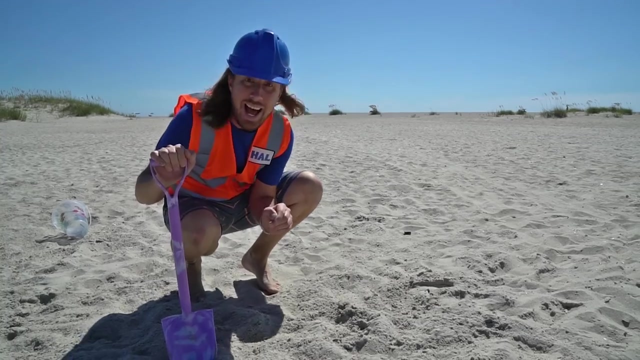 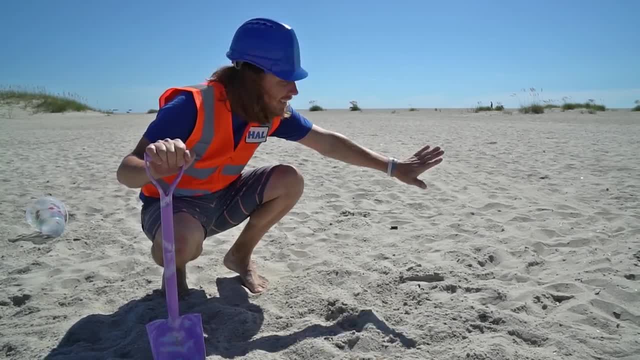 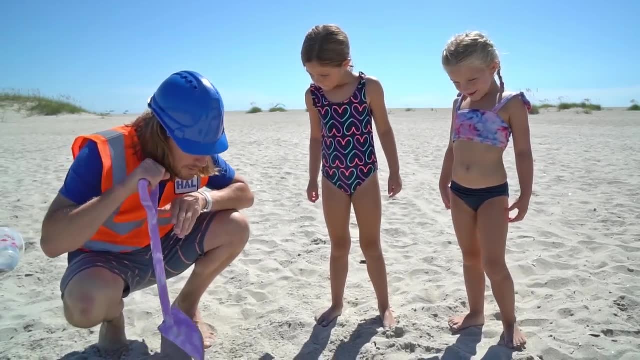 Kind of to protect himself. Hey girls, come look at this. Easy, easy, easy, easy quiet. If you look right there, you see there's a ghost crab in the ground, Isn't that cool? And he's kind of trying to protect himself. 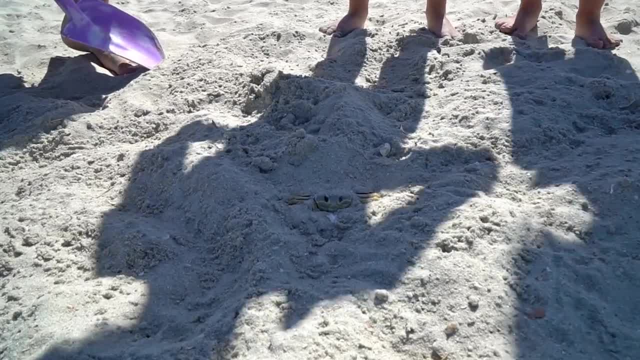 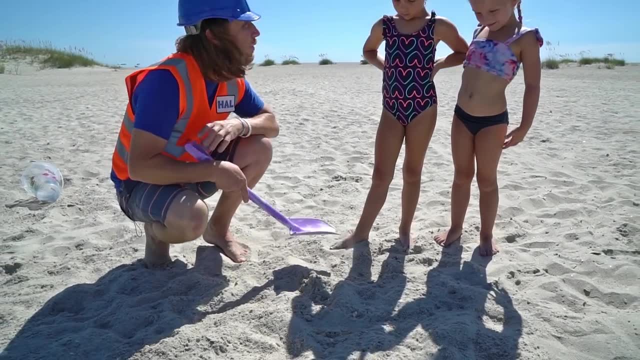 And he's buried himself down in the sand. Isn't that really cool? Oh yeah, You can see his eyes sticking straight up, You see it. And the rest of his body is in the sand. Let's see if we can try and move him. 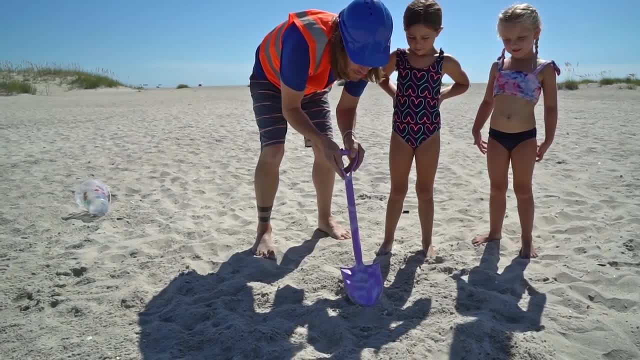 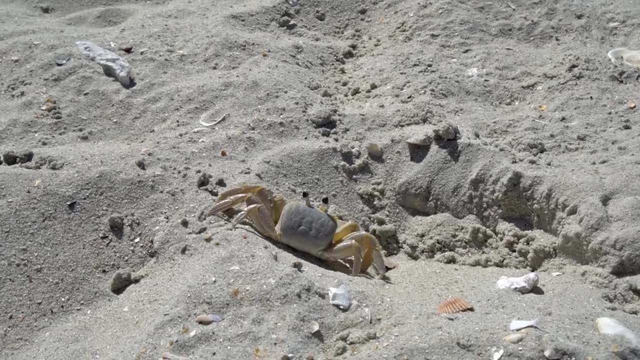 Alright, y'all ready, Here we go. Here we go. He's moved really really quick. See, Oh, there he goes. Looks like he found his home. That's awesome. Oh, wow, my friends, Being at the beach is totally awesome. 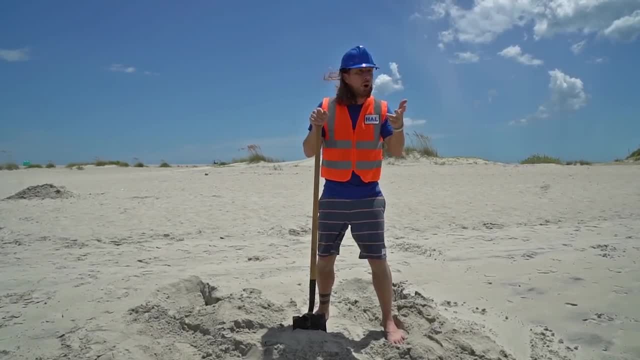 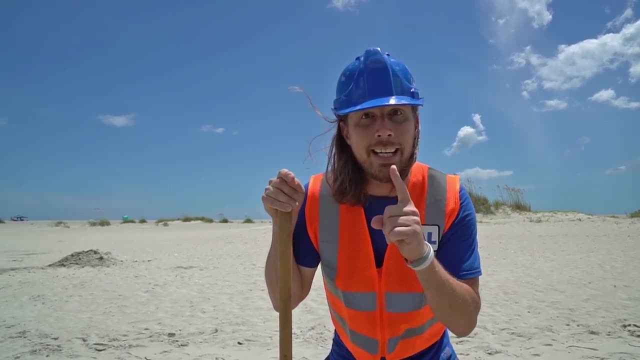 There's so many cool things to do, Like playing in the water, Surfing Or playing in the sand. Oh, you can build a sand castle like we did. There's so many awesome things to do. I think I got a really cool idea again. 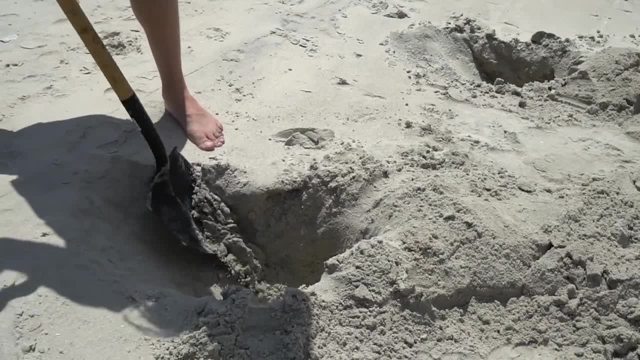 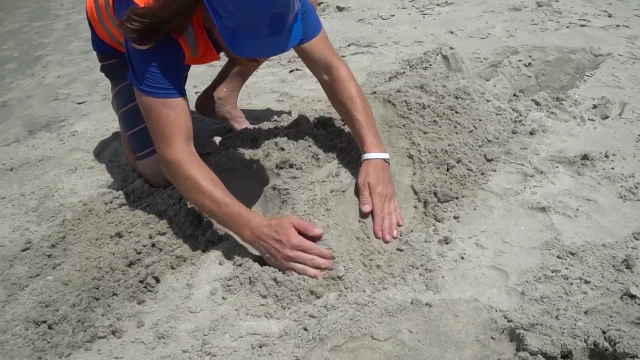 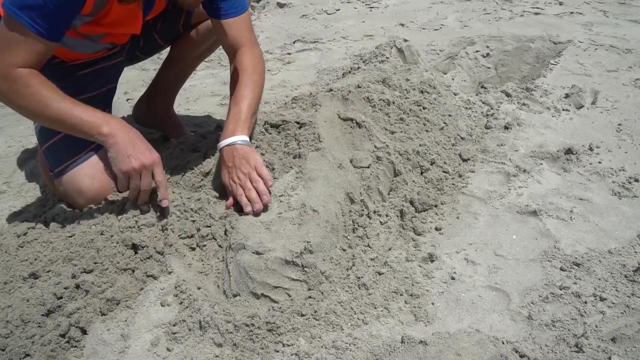 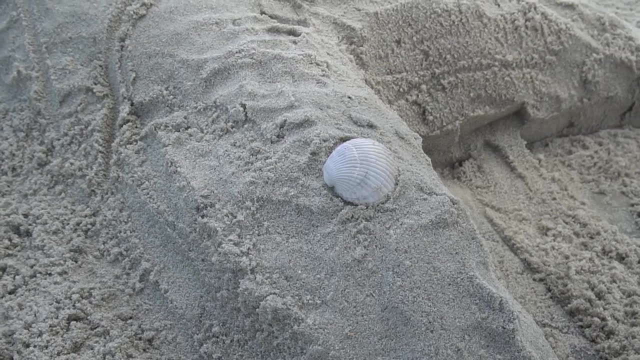 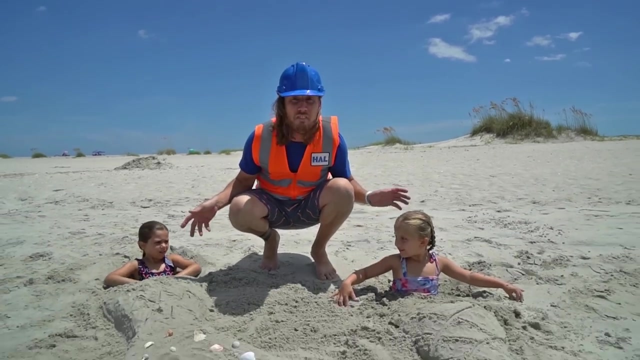 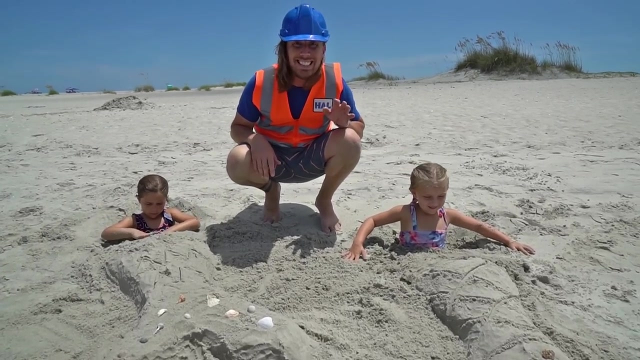 Let's go. Wow, look, I found a couple of mermaids. Totally awesome. We've had such an amazing day here at the beach In Pawleys Island, South Carolina. It's been awesome. We built sand castles. We found hermit crabs. 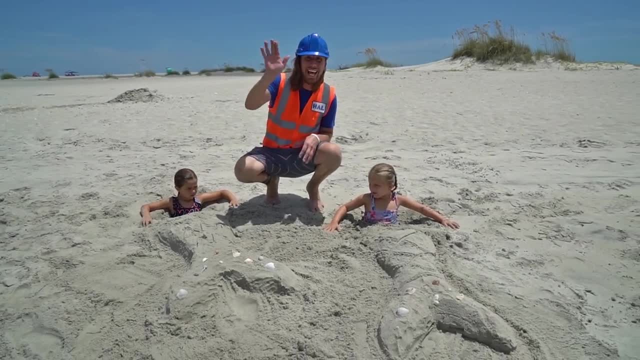 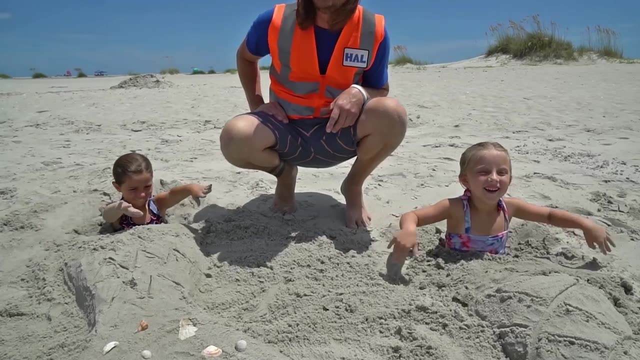 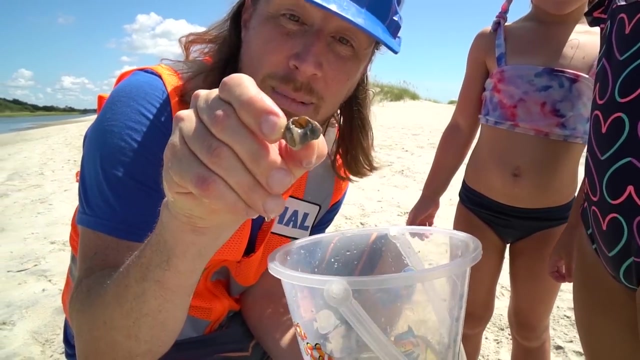 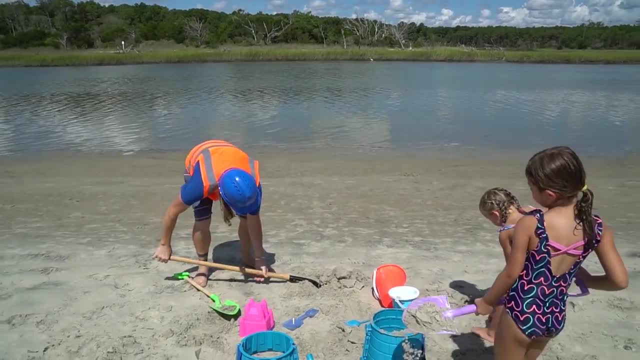 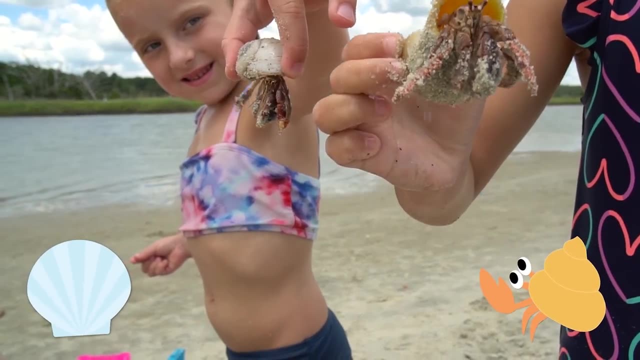 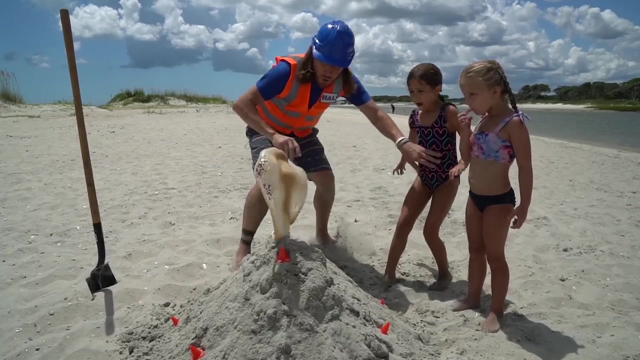 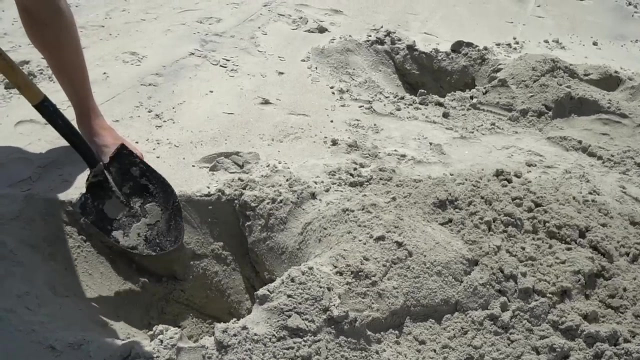 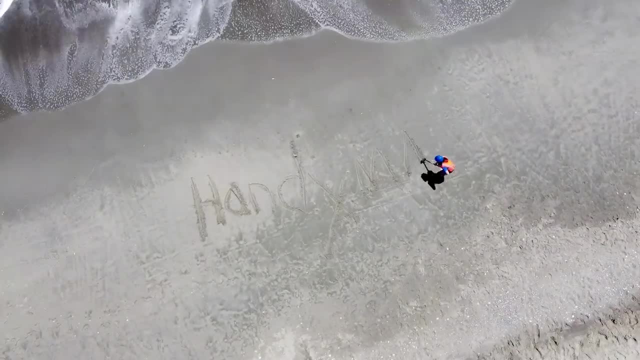 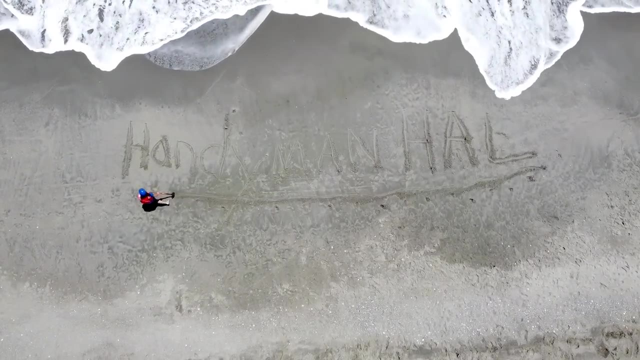 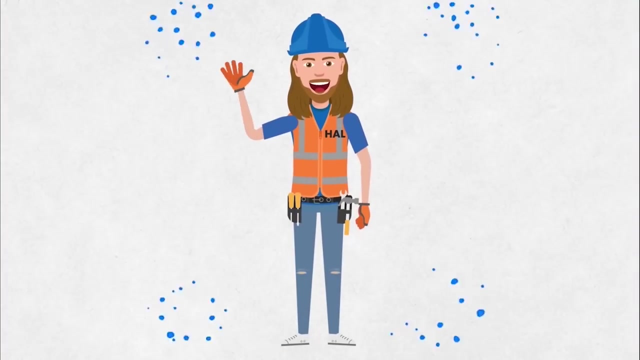 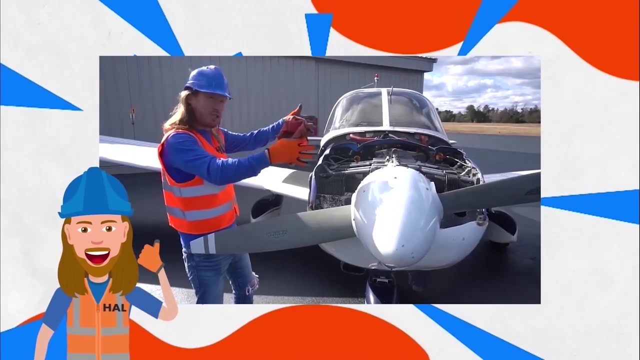 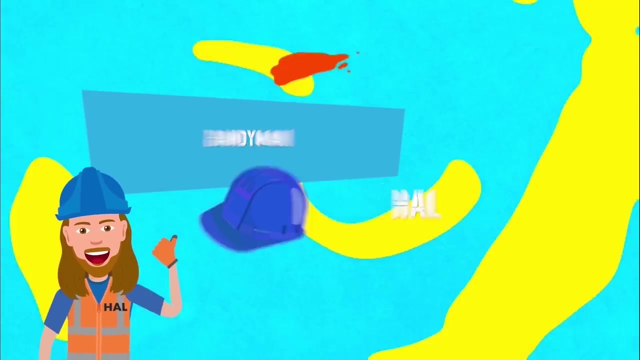 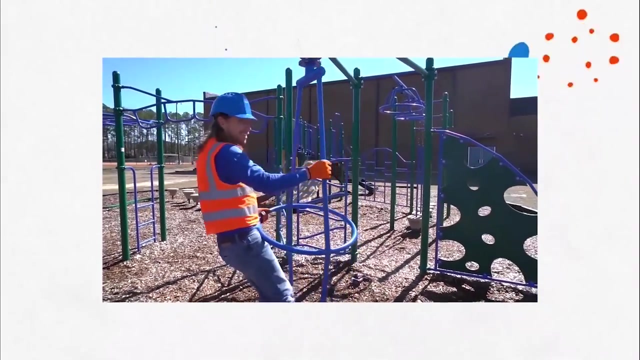 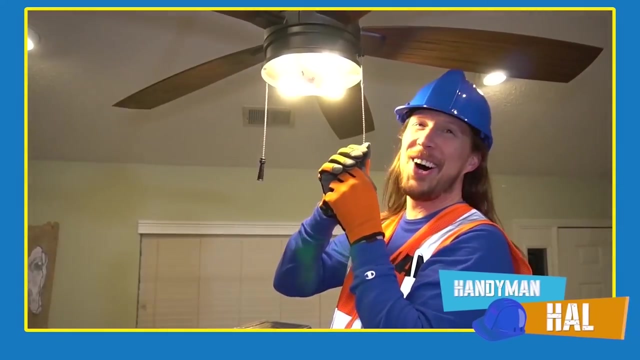